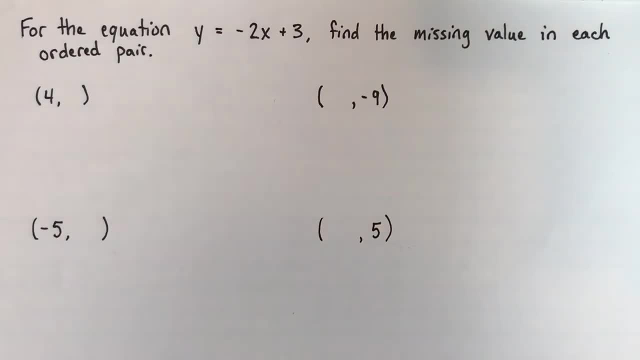 Hi, in this video I'm going to show you how to find missing values in an ordered pair, if you know the equation. So here we've got an equation: y equals negative, 2x plus 3, and we've got four ordered pairs and each of them is missing one value. 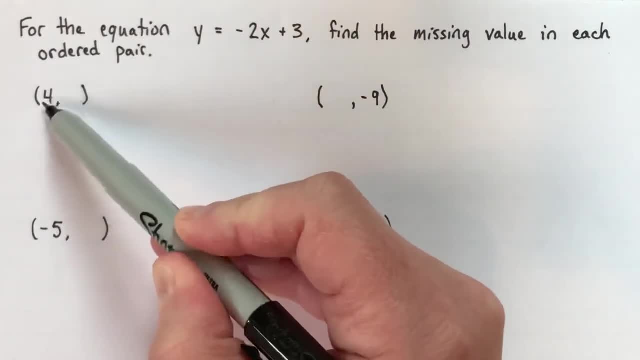 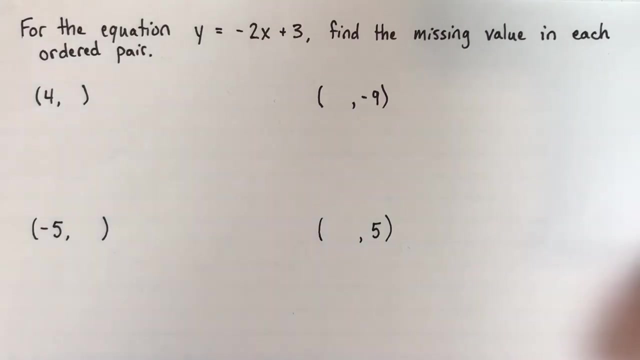 So if you notice the two on the left here, we know the first number and we're missing the second and the two on the right, we know that we're missing the first and we know the second. All right, so the concept here is pretty straightforward. I'm going to really try to. 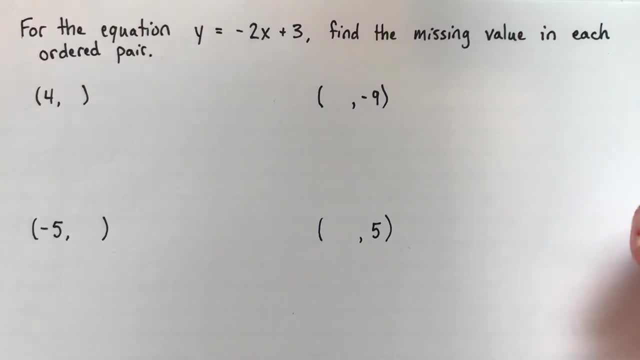 emphasize something that will help you avoid a pretty common error, and then you'll sort of see how it works. I'll go through all four examples. So the first thing you really need to know and remember is that, in an ordered pair, I'll write this here: you need to remember that the values 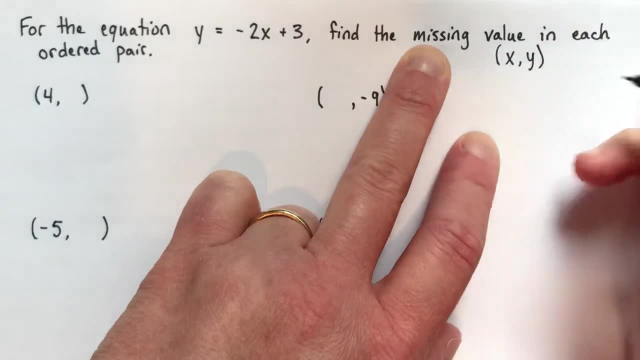 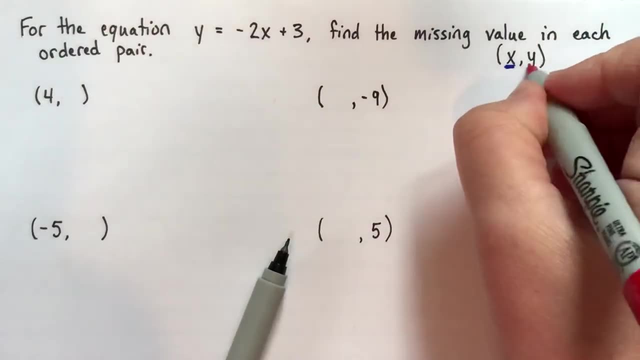 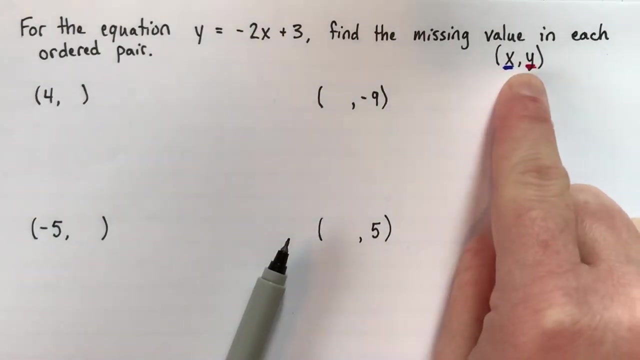 in the order of pair come in alphabetical order. That's super, super important And I'm going to actually even color code this- x and y- because it's so easy to make mistakes with this. This is the most common way people make mistakes. So the values in the order pair x comes first and y comes second. but in a lot of common 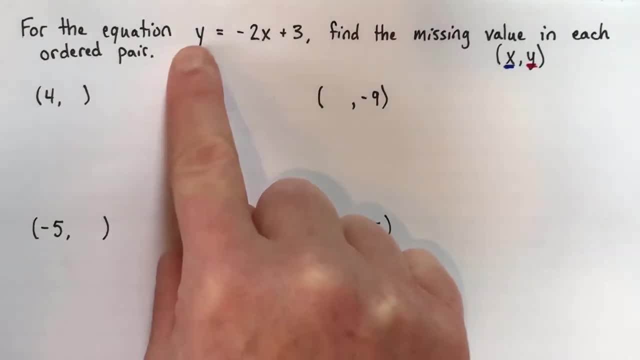 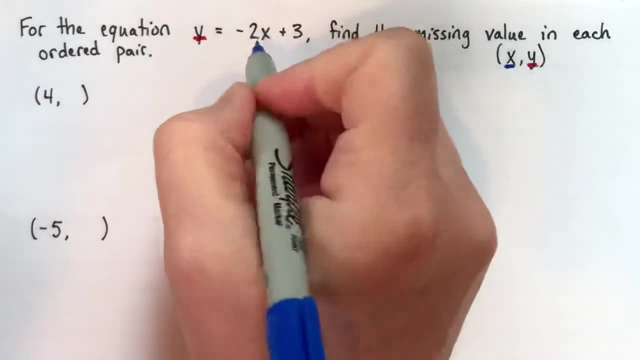 forms of the equations that we use, you notice that it's actually the opposite. so often- not always, but often- we'll have y come first in our equation and x come second. So you really need to just be careful, and I would encourage you if you're just learning the uppercase. 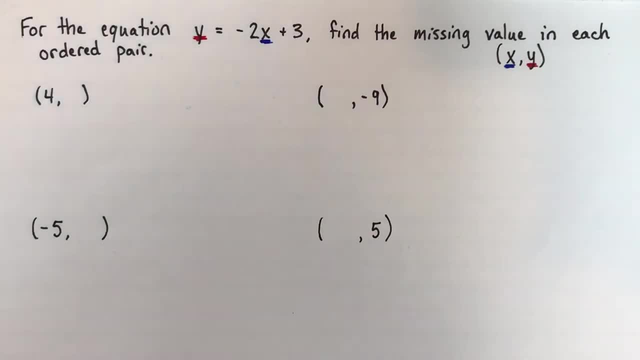 If you're just learning this or just reviewing it and it feels kind of new, I'd encourage you maybe to try color coding as well, not because the colors themselves are so important, but because it really forces you to slow down and make sure you put in the right values. 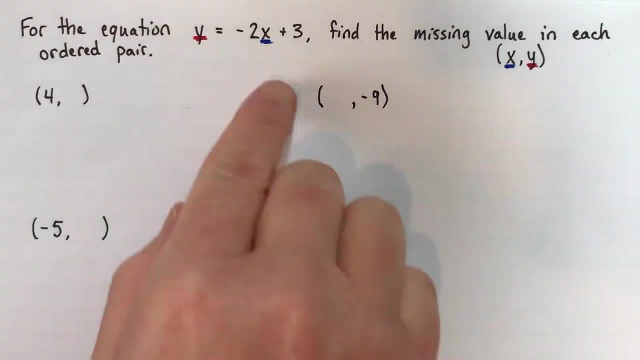 in the right place. All right, so let's start First. we have the ordered pair for something. So this, the first number, is our x value. So what I'm going to do is I'm going to substitute it into the equation and I'm going to make: 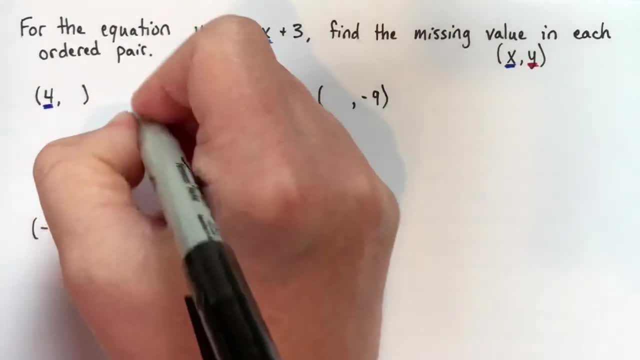 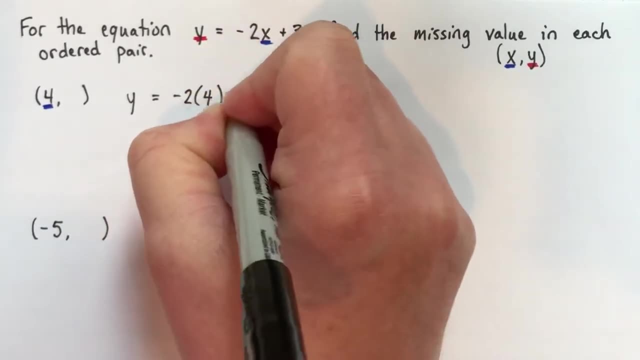 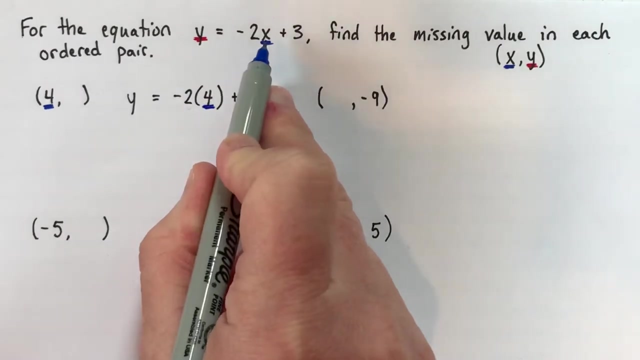 sure I'm replacing my x with 4.. So I've got y equals negative 2 times 4 plus 3. So that there is my x value right. So it was in the x position in the equation and it's in the x position in the ordered. 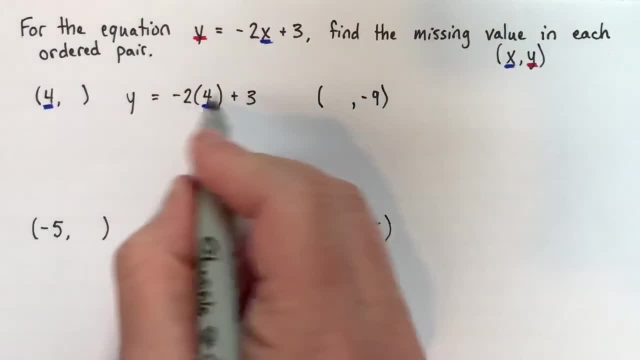 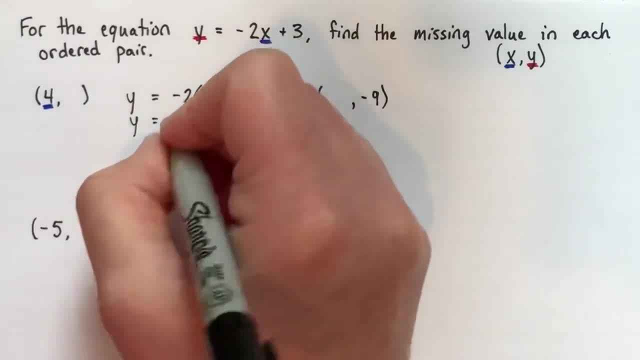 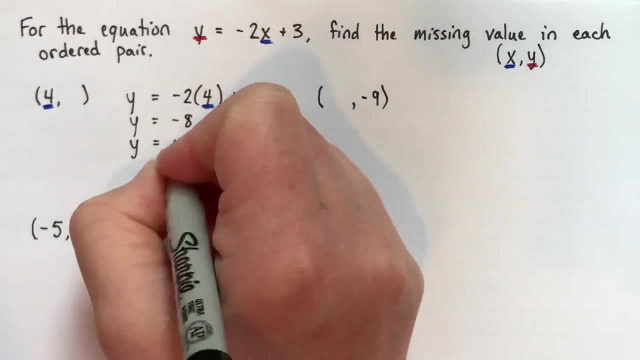 pair All right. so for this example it's just a question of simplifying. Okay, The next example will feel different, but here we've got y equals, all right. so negative 2 times 4 is negative 8 plus 3, and negative 8 plus 3 is negative 5.. 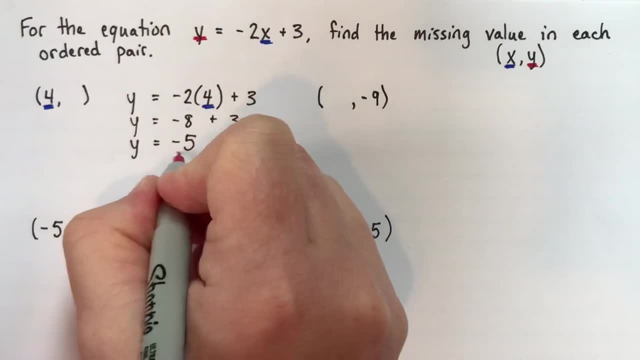 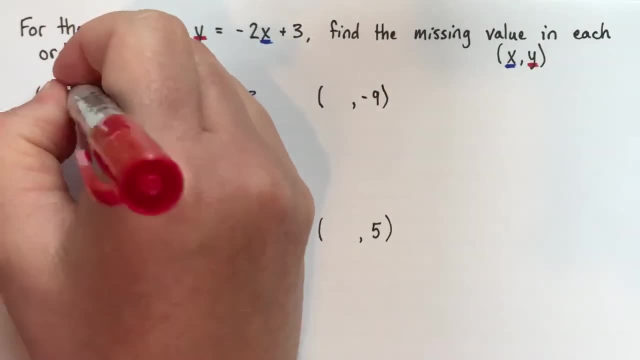 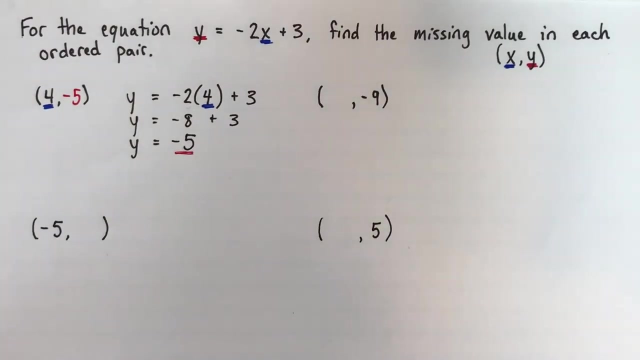 All right, so that is our y value, because it says y equals negative 5.. So it goes in the second spot in the ordered pair. All right now. I want you to pay attention to this. I want you to pay attention to how different this next example will feel. 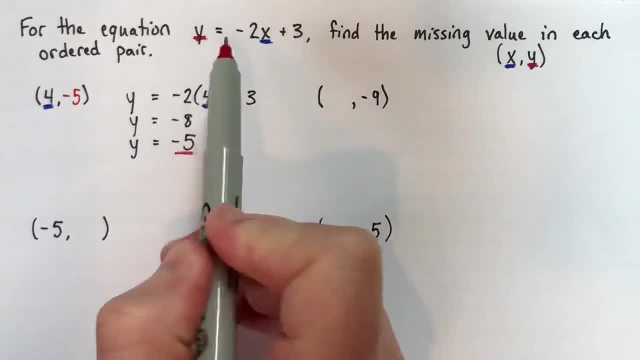 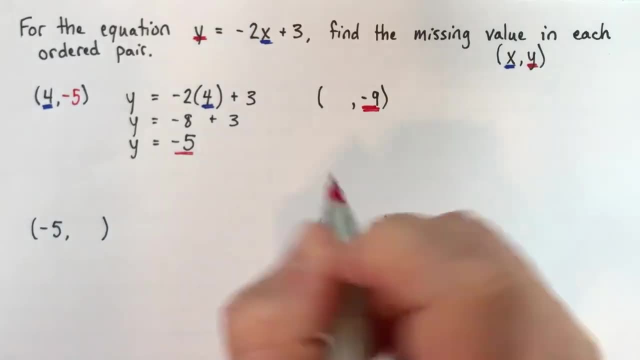 The concept again is the same, but there's something about the way the equation is written that makes it feel different. So negative 9 here, that's the second number. so that is our y value. So when I write my equation I'm going to replace y with negative 9, and that is equal. 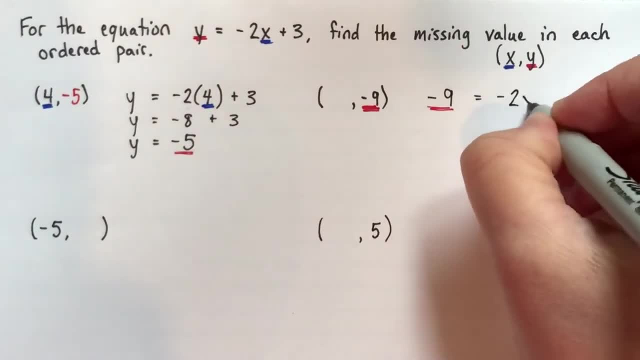 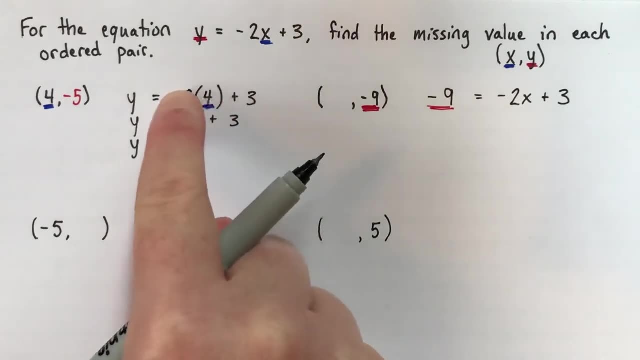 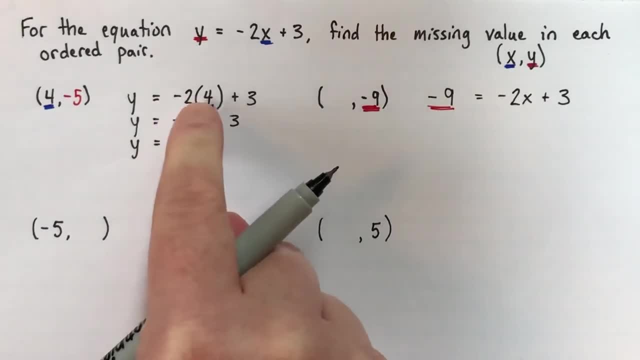 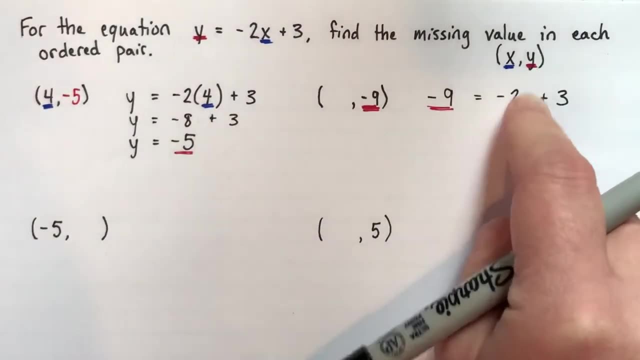 So we just had to do that little calculation, Made sure we followed the order of operations, but there was no real other trick to it. Here we're looking for the value of x, but x is sort of in the middle of this. the right. 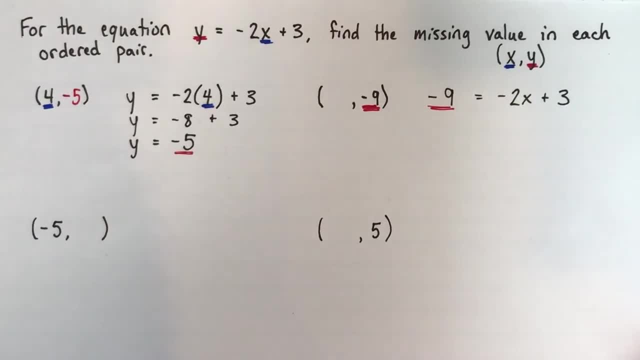 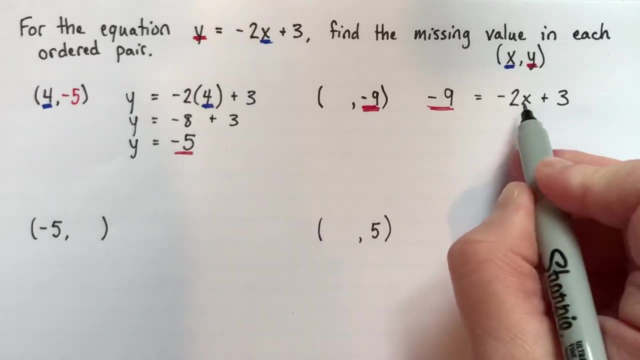 side of the equation here and there's all sorts of other numbers going on. So we're going to have to solve this equation here. So we're trying to isolate, We're going to isolate x to figure out what the missing value of x is. 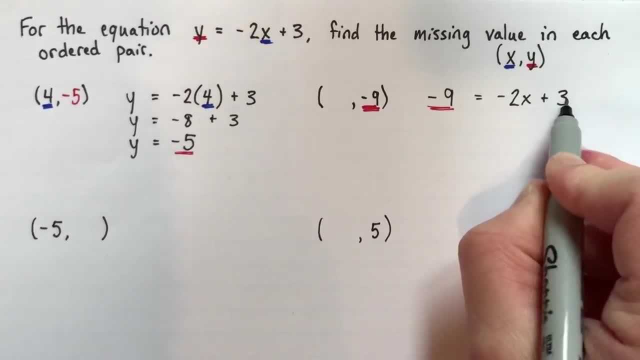 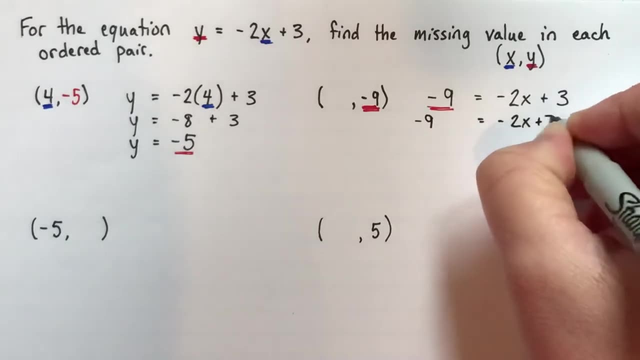 So we look at this equation, We've got negative 2x plus 3.. So what I'm going to do first is I'll subtract 3 from both sides, I'm going to write the equation again, and then I'm going to subtract 3.. 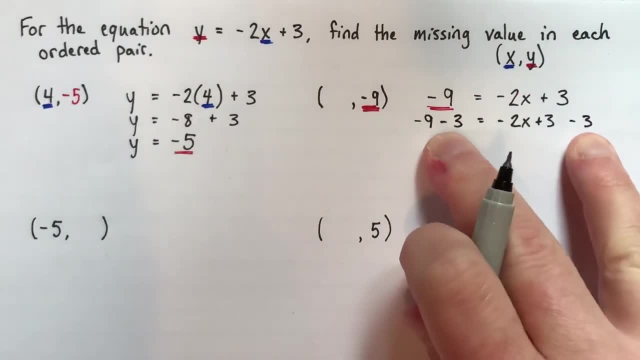 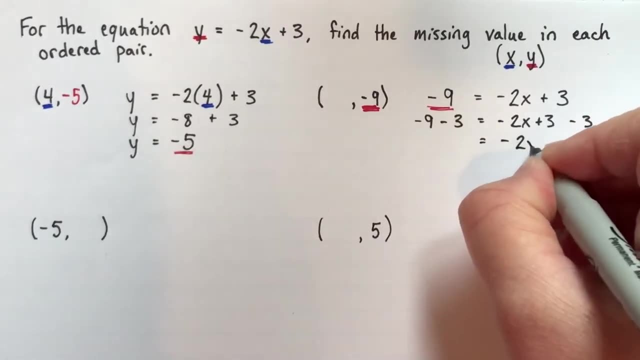 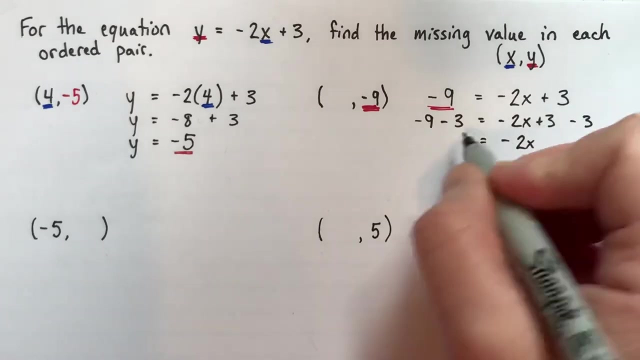 And to keep both sides equally the same, I make sure I do it at the same time on both sides of the equation. So on the right that gives us negative 2x. That was why I did it All right. I subtracted 3 to sort of make it feel like I was getting rid of this plus 3.. 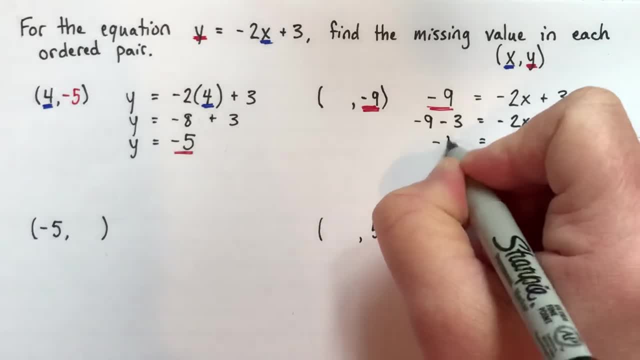 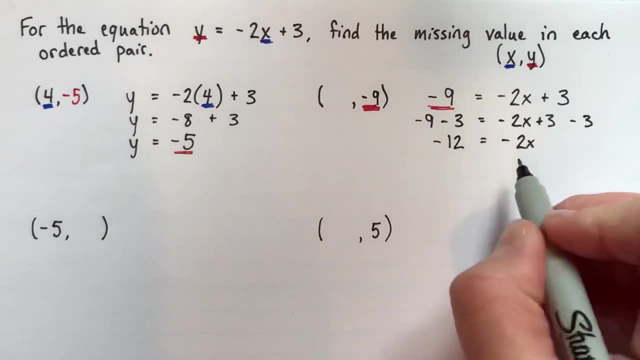 And then over here negative 9,. take away 3, is negative 12.. All right, Now there are several ways of dealing with this negative 2 here, but I think the quickest if I've got negative 2x and I'd like to just have x, x times negative 2,, so I'm going to 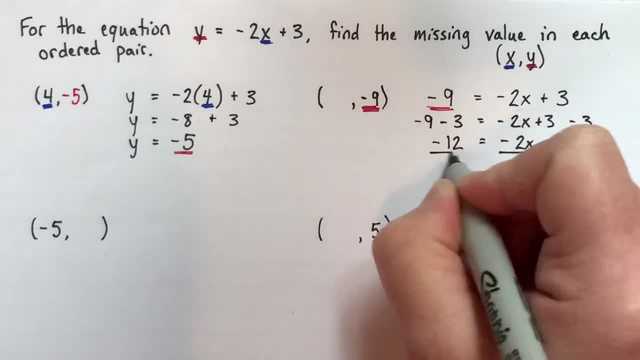 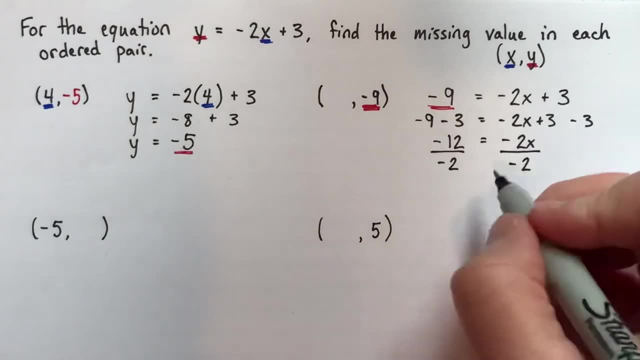 divide by negative 2 on both sides of the equation. Because multiplying by negative 2, I'm going to divide by negative 2.. Because multiplying by negative 2 and dividing by negative 2 are opposites, so they undo each other. 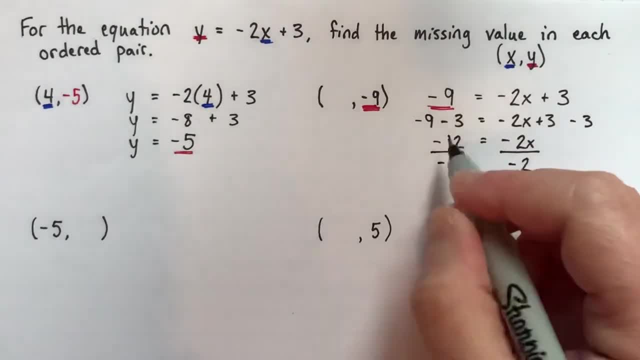 All right. So on the right, that gives us x And negative, 12 divided by negative 2 is 6.. All right, So here is our x value. x is 6. And so that means the missing value here is 6.. 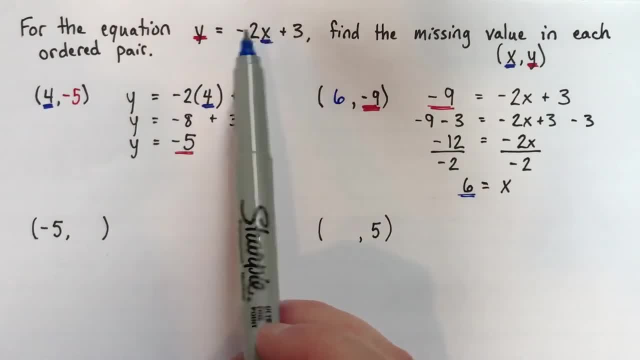 All right. So just because the way the equation is written, where y is isolated in the equation, if we replace the x value, it feels much more straightforward to just calculate. But if we replace the y value when we're looking to find x, we really have to solve an equation. 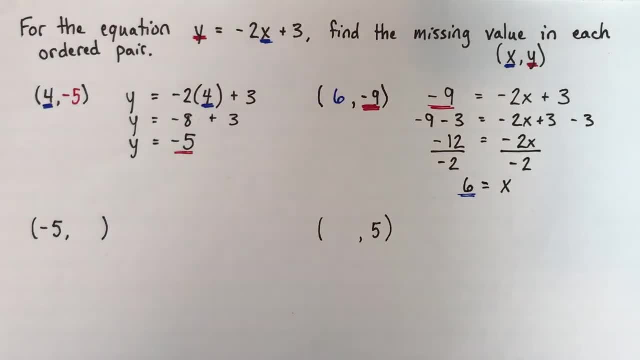 algebraically here, All right. So I'm going to do one more example of each. I'd encourage you maybe to pause the video and do this calculation on your own and then watch me go through it to see how you did. But obviously you can do what is right for you. 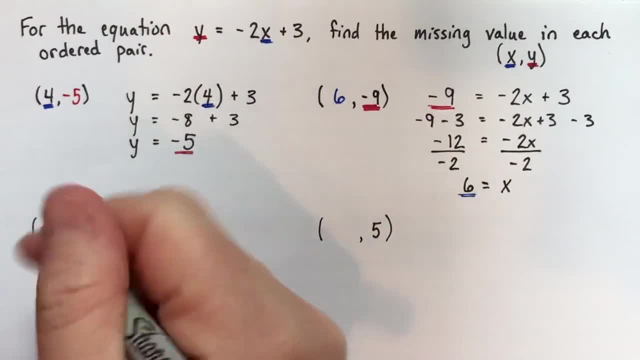 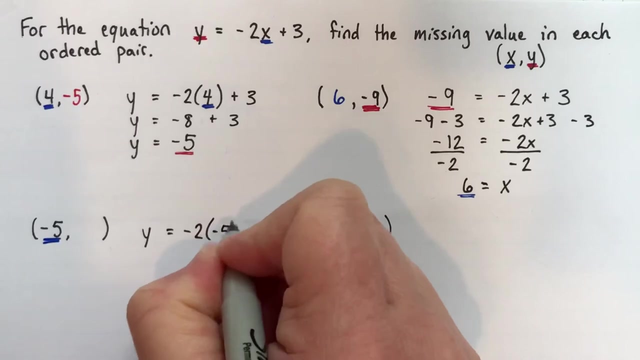 So here is negative 5.. That's our x value. So I'll copy the equation and I'll replace my x with negative 5 when I get there. So y equals negative 2 times negative 5 plus 3.. So here it's just a question of multiplying and adding carefully. 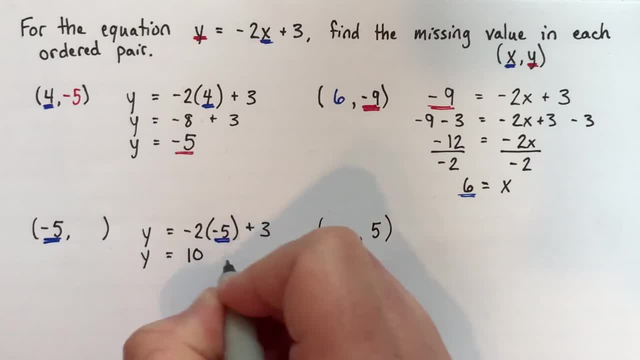 Negative 2 times negative, 5 is positive, 10.. All right, So negative 2 times negative, 5 plus 3.. And that's 13.. So that's my y value. So the missing number here for y is 13..